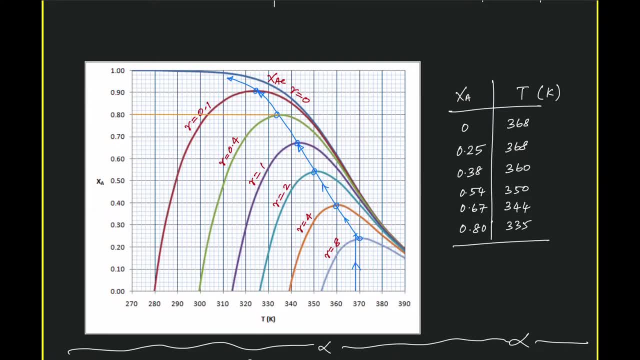 what we are interested. We change. we have this range of temperature, So we need to find the optimum temperature So as to cover the inlet feed temperature. Now, inlet feed temperature is given, which is 3- what is it? 95 degree Celsius, So the operating temperature will be starting from this inlet. 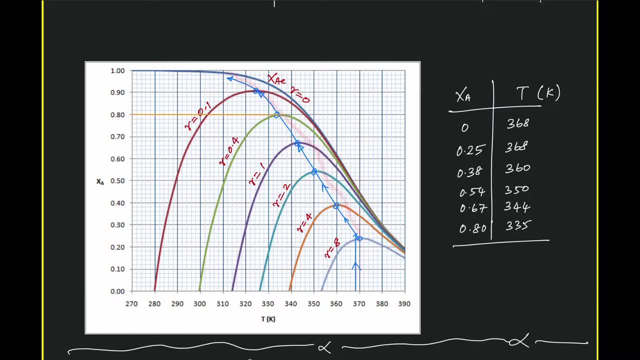 temperature. the operating temperature is normally lesser for the reversible exothermic reaction. That's why I am covering this range from 270 to, say, the maximum of 390 Kelvin. So what we are going to do, we want to get the plot of XAE versus temperature first, then, for various rates, we want to get the plot of XA versus. 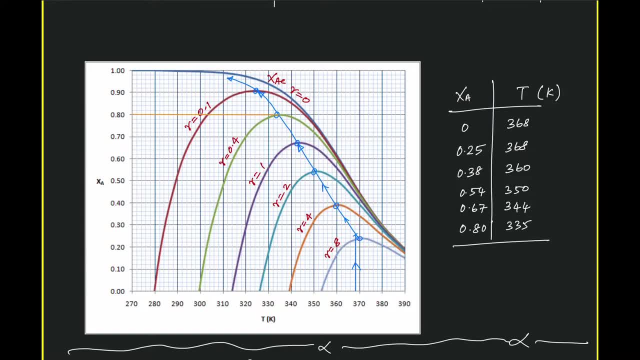 T. So what is the need for that? because we want to get the points. or is locus of these points? These are nothing but the maximum of these rates, So we want to get these line. that is a final one, what is called as a optimum temperature progression. 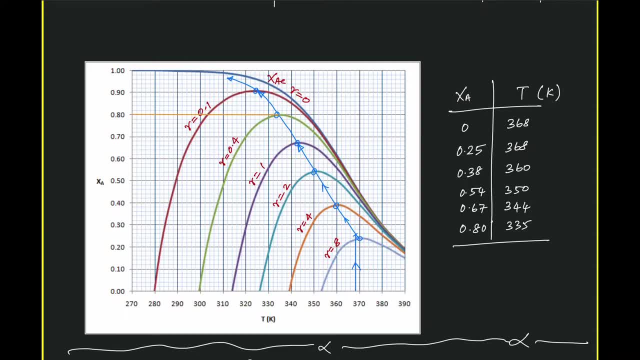 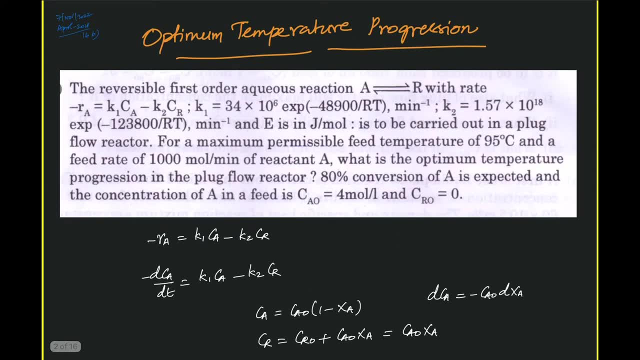 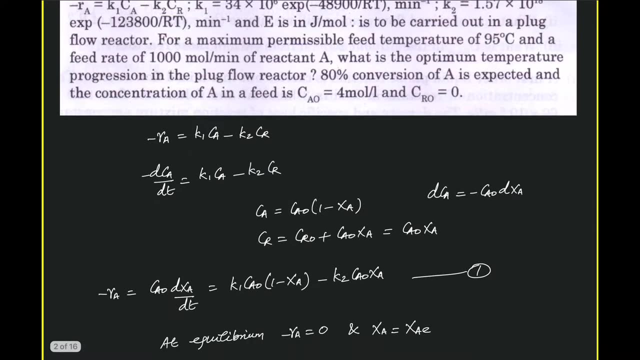 So to obtain that. but what we have done, let us see so, for the reaction is already. rate expression is given and we can also write this rate in terms of conversion minus dca. byte T is equal to. of course, dca is equal to CA naught minus CA naught into dxA, from which we have DCa by Tt is CA naught into dxA. 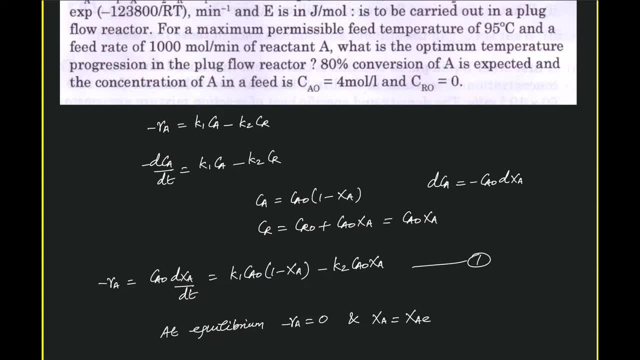 Now to get the sample for the reaction you come to these, let's try and write this inverse expression in this penultimate approximate equation, which is caracterized of equal to ah minuseter XA minus RO2O, by Tt. to Tt, that is equal to DCa to circuit breaker, DCA minus CAoc, into dxA, into Cha, from which we have DCa. by Tt, is Ca naught factors here. so for Vgesh AS is igual to buddy ballario. 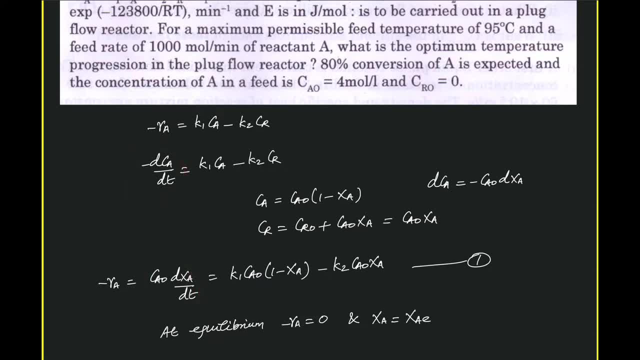 a naught into dx, by dx, a by dt and ca, is c? a naught into 1 minus x a. cr equal to cr naught plus c a naught into x a. of course r is not there, so we have only c a naught x a. so now 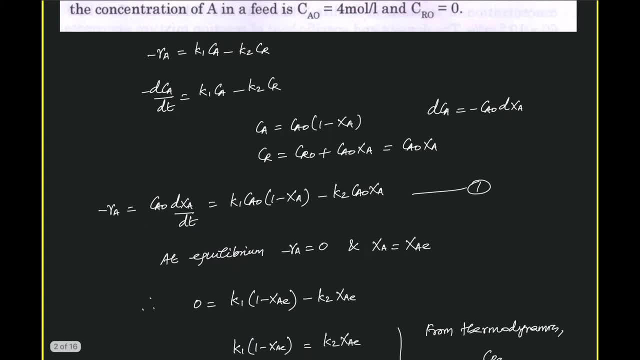 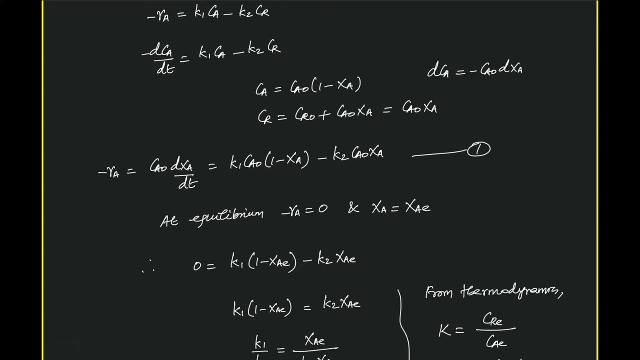 this expression is available in terms of x a, c 1. sorry, x a, k, 1, k 2. so k 1, k 2. already we have the expression in terms of temperature and what are all available. so, okay, we have k 1 and k 2 as a. 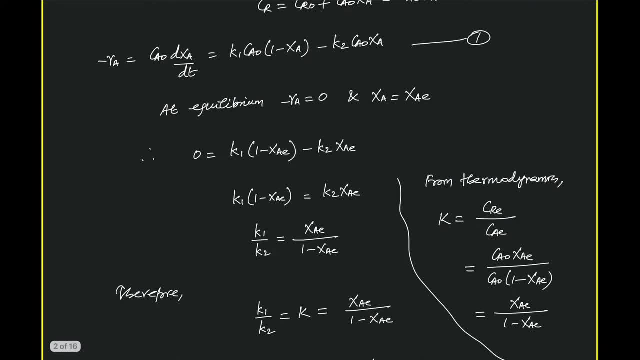 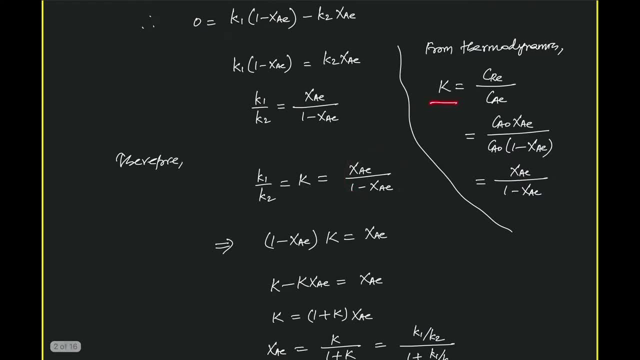 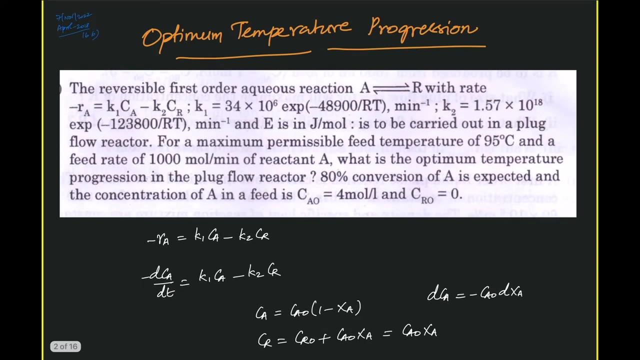 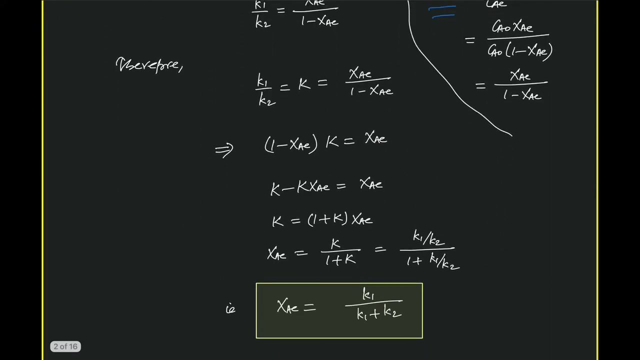 function of temperature. and additionally we can also write this x a, e from equilibrium conversion, equilibrium constant as well, of course, which is not needed now because directly we have this k 1 and k 2. so that is enough for our problem, because now this x a e 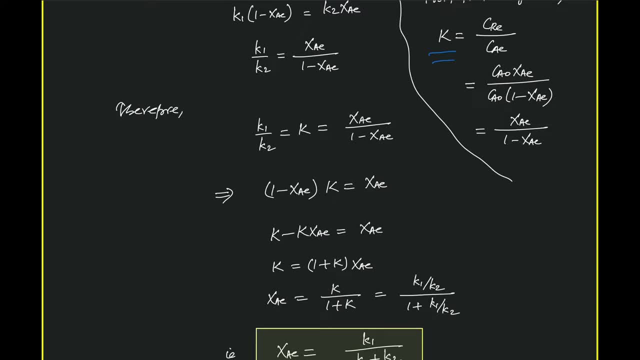 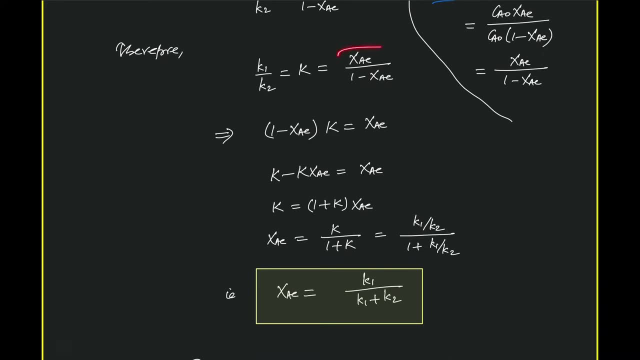 for getting this equilibrium conversion we need this k 1 and k 2 values, so k 1 and k 2, otherwise you can rearrange this expression and this can be this: k 1 by k 2 is x a e by 1, 1 minus x a e. otherwise x a e can be written x a e equal to k 1 by k 1 plus k 2, or simply. 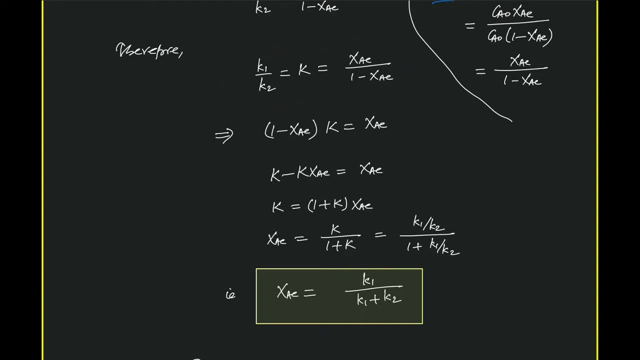 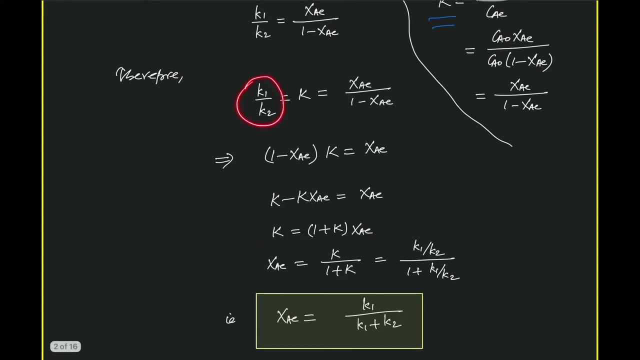 rearrange this part. of course we need not worry about this capital k, which is also coming at this. k 1 by k 2 is also coming as capital k, so otherwise there is no need for that. simply you can write this x a e directly from this: values of k 1 by k 2. so x a e equal to. 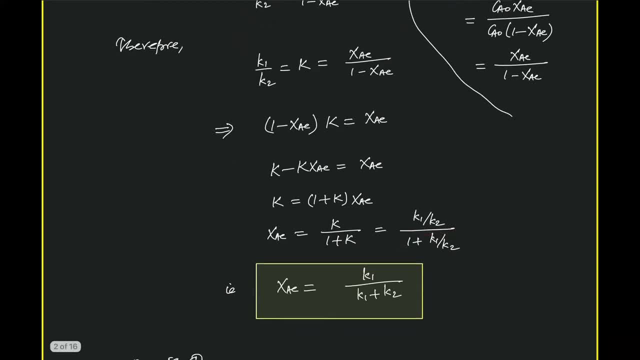 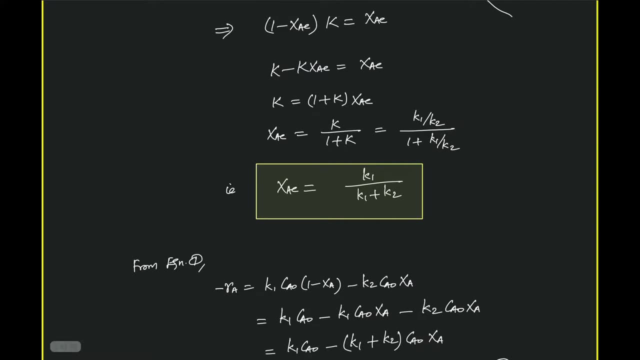 k 1 by k 2 by 1 plus k 1 by k 2, 1 by 1 plus k 1 by k 2, so from which we have this final expression. so what are all known to us now? already we know the expression of k 1 as a function of temperature, and 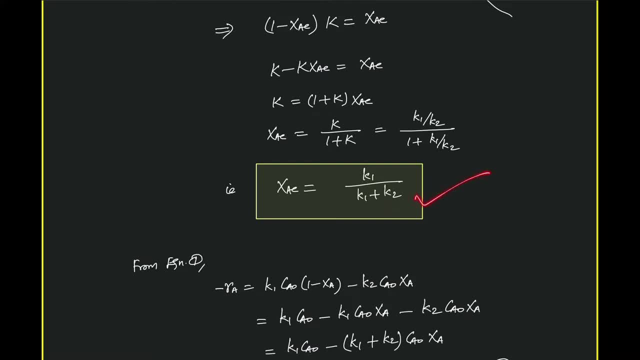 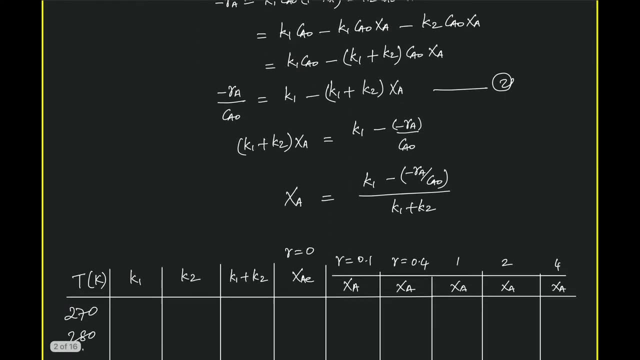 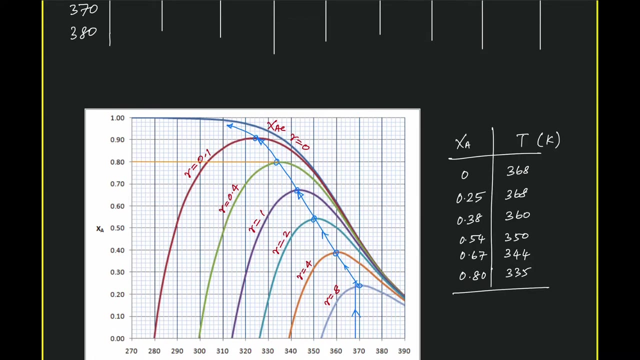 k, 2 as a function of temperature. so x a, e as a function of temperature, is can be easily obtained. additionally, what is needed is: we want to get otherwise, what is now available is this: the data for this curve is ready. in addition, and now we want this, graphs generated otherwise, for 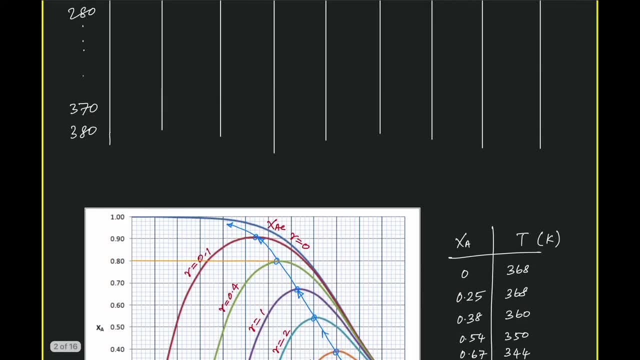 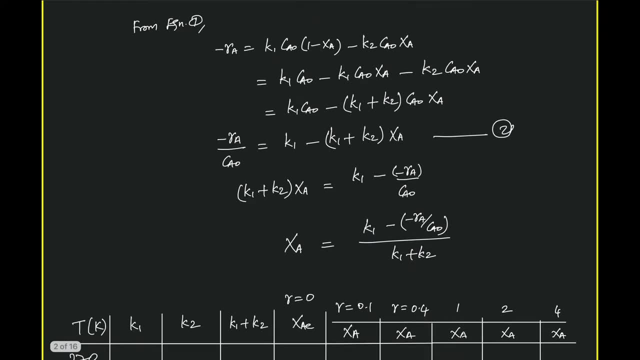 every rate. we want x, a versus t. so what? what we are going to do? again, from the rate expression, from the rate expression, we are rearranging to the form that xa as a function of k 1 and k 2 for a given rate. so now what we are going to do? we are fixed. we are going to fix this rate. 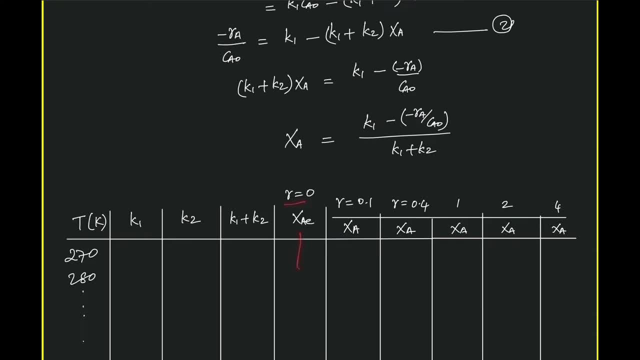 to some value, say starting from 0. already we have this is equilibrium conversion. we are going to fix this rate for some function in the left side. so x a e plus k 1 by k 2 says into k 1. we are going to achieve this equation and that is: k 2 is equal to i by 1 plus x a e minus k 2 by k 1 into k 1 by k 2 is equal to x a e, even equal to k 1 plus k 2 by k 2, wants to be given accordingly. 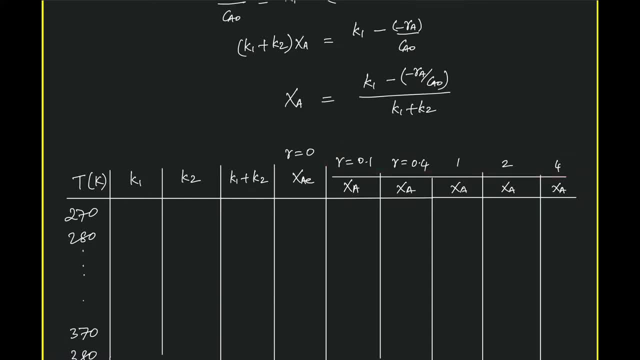 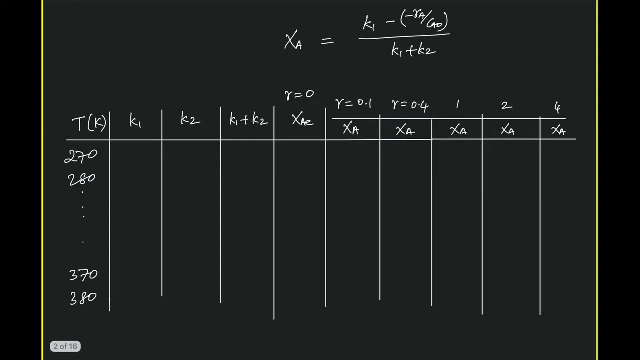 some positive numbers, of course. what number? to choose this? again, if we have this excel program readily available, we can easily construct a table and take some values of r for each and every r. we can get this xa and we can easily make a plot and we can always idea of telling this is we are going. 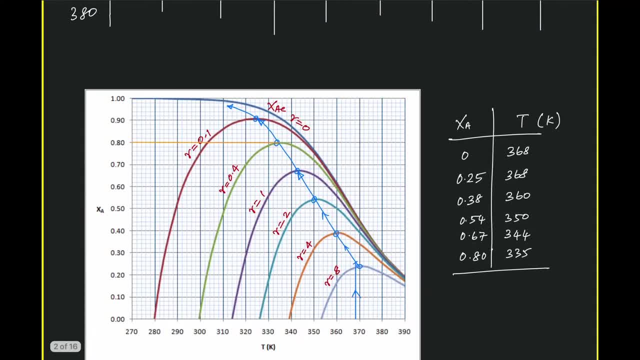 to choose a rate value so that we are getting a plot like nice plot, in the wider range of temperature, of course, for various range of temperature, or if it's for this range of temperature. we want to get these plots. so initially i am assuming point one, so i this: 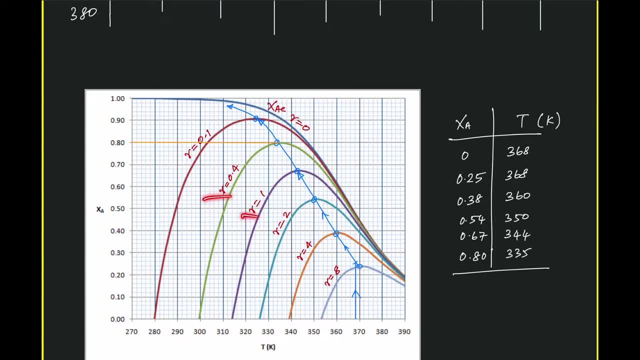 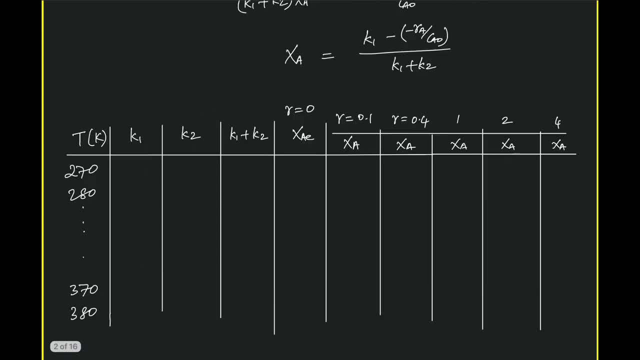 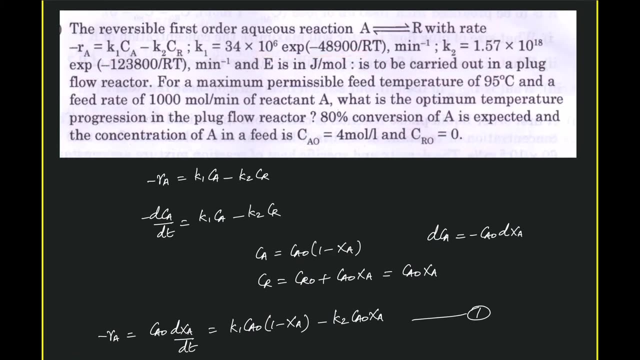 nice plot is obtained. likewise for other rates. we are getting this. xa values say k1, k2. we have to obtain how to obtain k1 and k2. we have this expression. in this expression, r has to be in the units of joule per mole. why it is to be? because this is given in joule per mole. that is the meaning of. 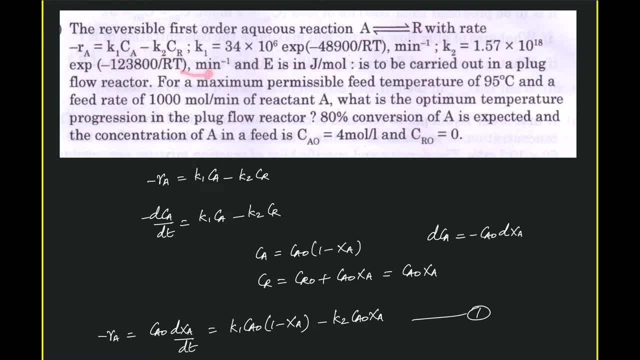 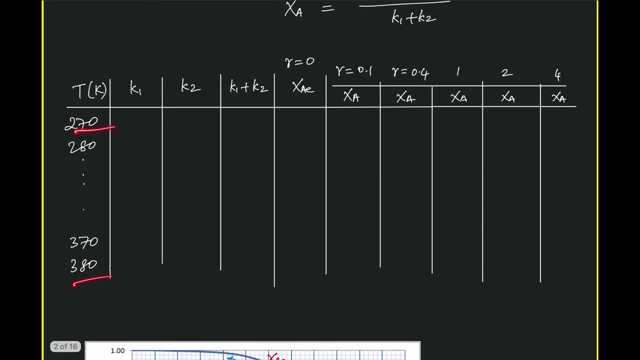 this statement, and temperature has to be in kelvin, and so k1, k2 are estimated for a range of temperature starting from 0 to, say, 110 degree celsius or so, so always for this range of temperature in kelvin. i am getting these values of k1 and k2 from the expression. 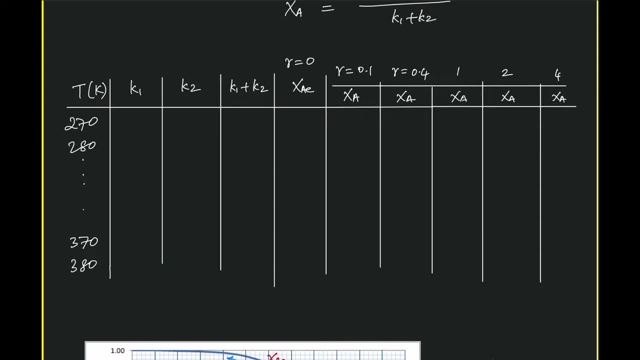 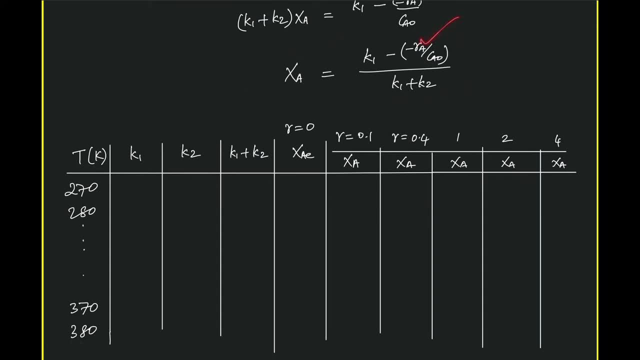 of k1 as a function of time and k2 as a function of time, then in in this expression, what is needed is for rate of zero. already we have obtained for rate of 0.1. choose a value of 0.1, of course. c a. 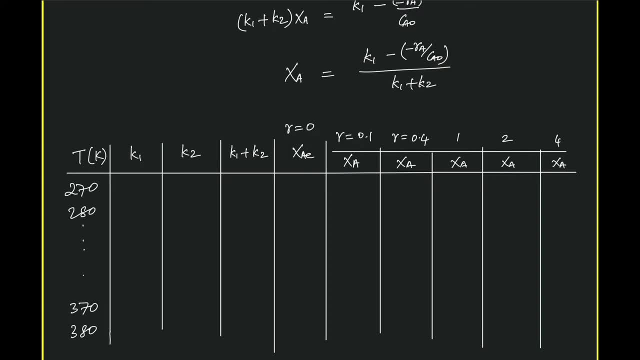 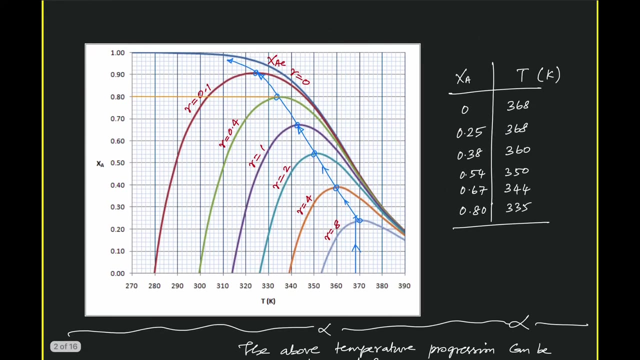 not, is given and we can, using this k1, k2 and k1 plus k2, we can get x, a, e, so for various values of assumed values of rate. so now the plot is obtained. there is, whatever the data obtained in this table is plotted here. of course i have plotted this. 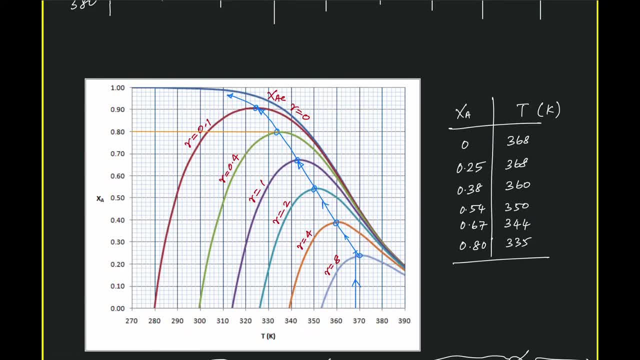 using ms excel, microsoft excel here. okay, these plots are nicely drawn now. so what is needed is we need to find the locus of maxima of these rates. so, locus of this, maxima of these rates. so, uh, you have to connect always. simply make a note of these maxima points and simply join them. 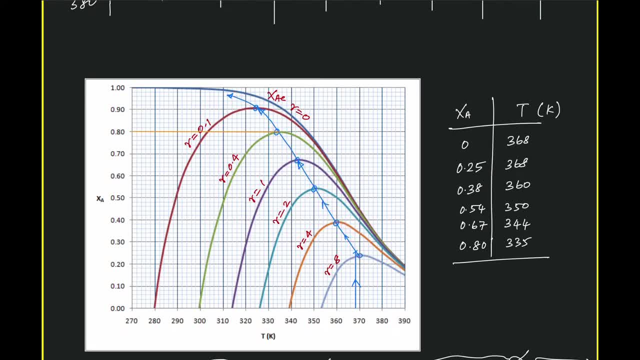 nicely. so this is what is giving. this is a conversion versus temperature plot. so, always, this is a conversion versus temperature data taken from this, this blue line, this is what is the optimum temperature progression starting at the 95 degree celsius. say, that is, 368 kelvin till. 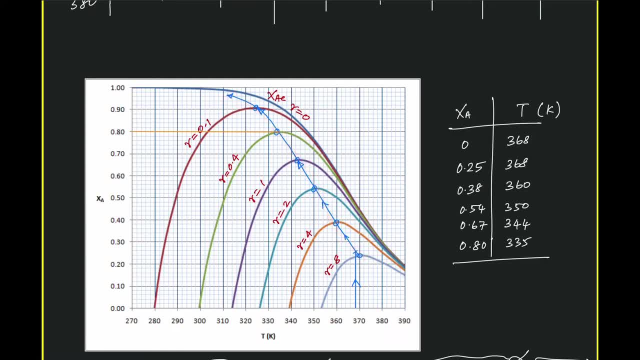 or this. this line is already drawn and this line is vertical line is drawn and the intersection point. from this point onwards, there is a reduction of temperature. till then we are operating at the maximum temperature. why it has to be reduced, or is why the temperature has to be reduced? then, if the 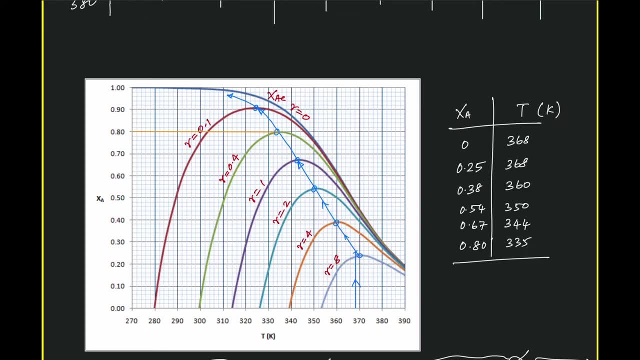 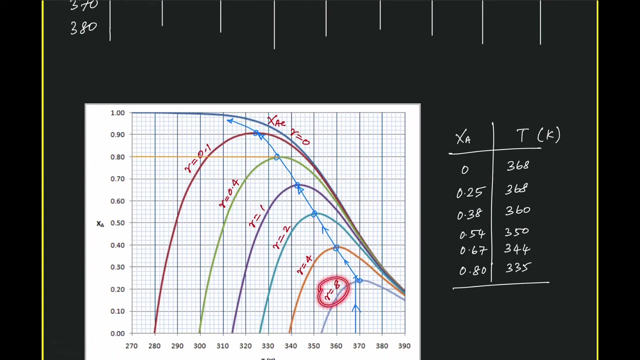 temperature is not reduced, then the conversion will go down. otherwise, if you simply operate at this temperature, along this temperature, isothermally, then after this point, rate is reducing, reducing, reducing. it is ultimately reaching to value of 0, whereas we need to have higher conversion, not only the rate, of course, conversion is also to be here. we could, if you can, keep keep on operate on. 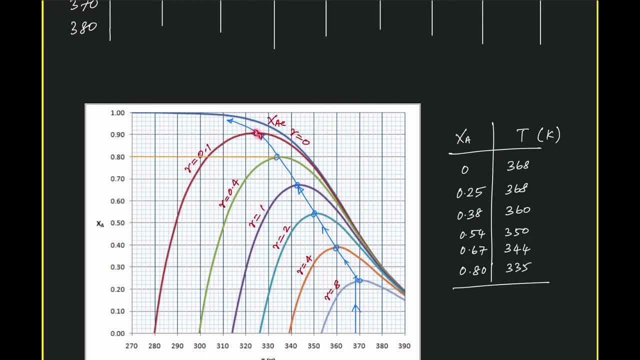 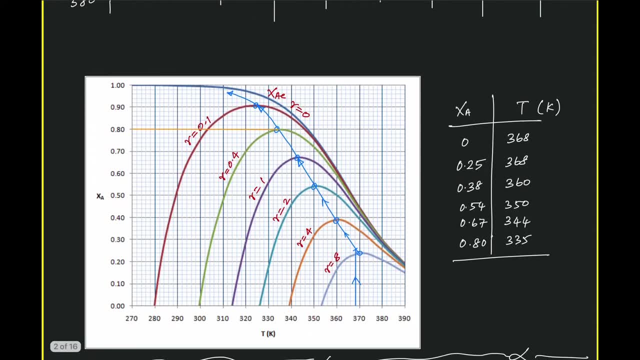 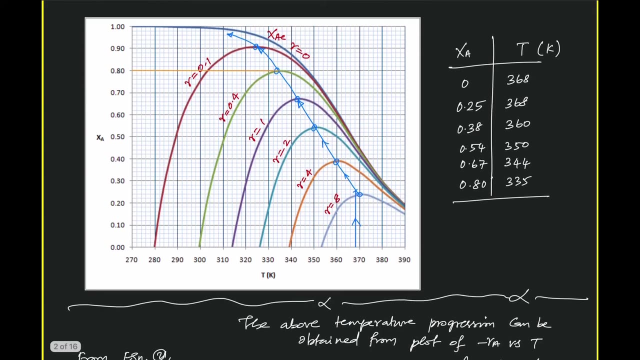 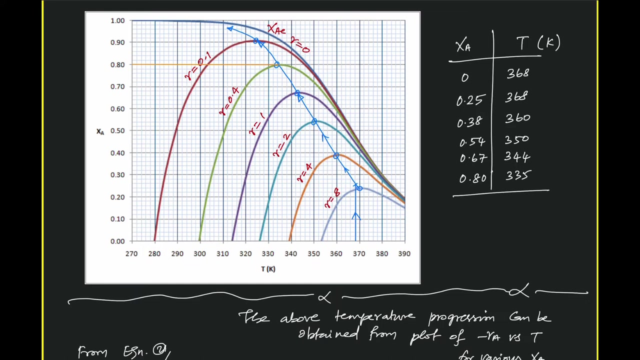 this temperature line. we can reach a conversion even to this level. so this optimum temperature progression is, uh, the locus of maximum rates for a given conversion. otherwise, say, here we have not very nice data. in what way? because suppose you are interested in getting what is the temperature for? 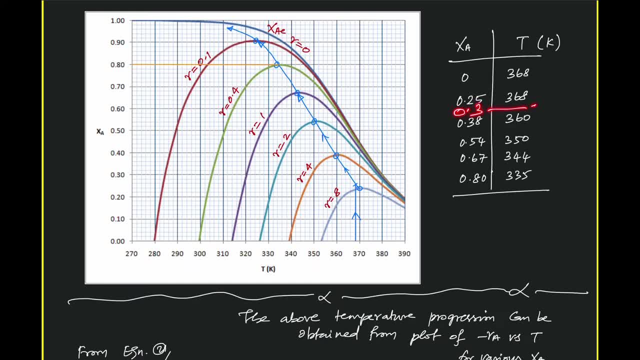 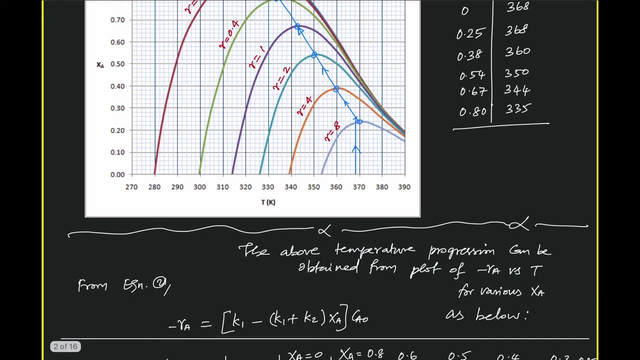 a conversion of, say, 0.3. i don't have this data directly from the plot, from the this table. of course you can interpolate, or suppose i am getting interested in getting the value of xa for xa of what is that t? for xa of 0.7, what is that t? so in that case, what we can do again, we can go back to. 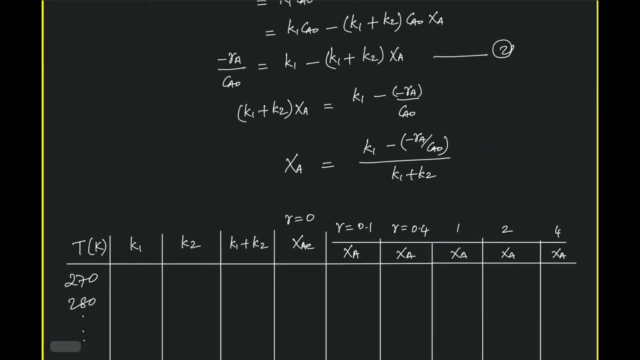 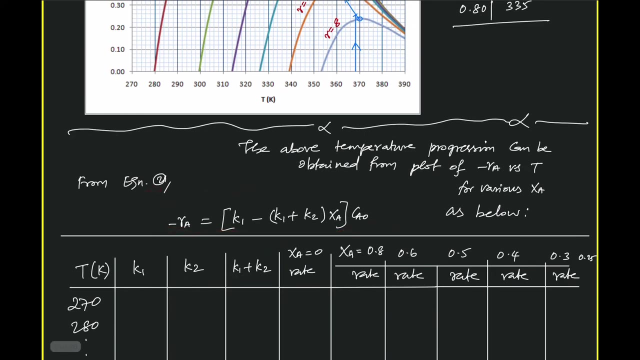 the same equation. so this equation we can rearrange in such a way that you keep xa as the parameter. i will skip xa at constant get a relation between r, a versus t. so otherwise we are rearranging the equation in such a way that xa is kept constant and for every temperature we have this k1, k2 for that every temperature. 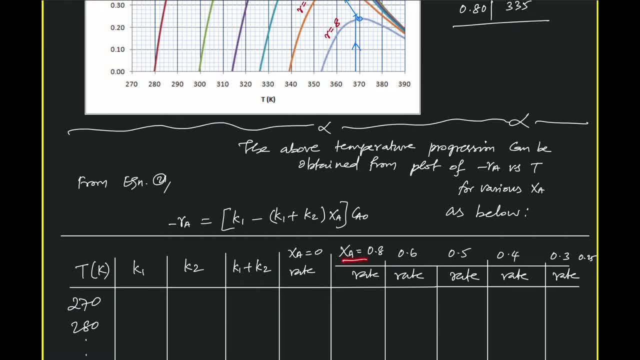 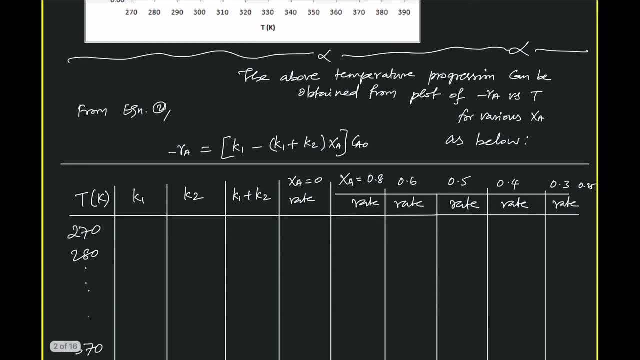 we are getting rate otherwise. at uh, every xa we are getting rate as a function of temperature. so this temperature k1, k2- already- these values are already available to us- and this xa equal to 0- that also we can get this rate data calculated simply. xa equal to 0 means okay, we have only k1 ca. 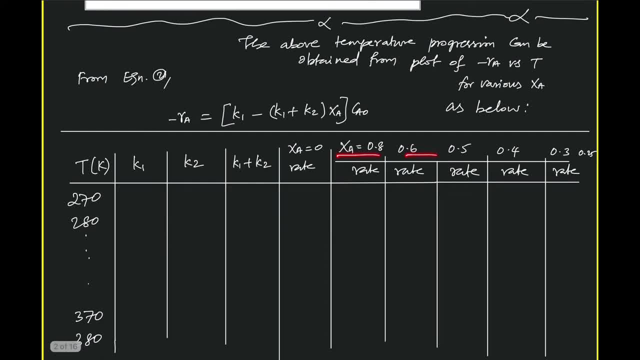 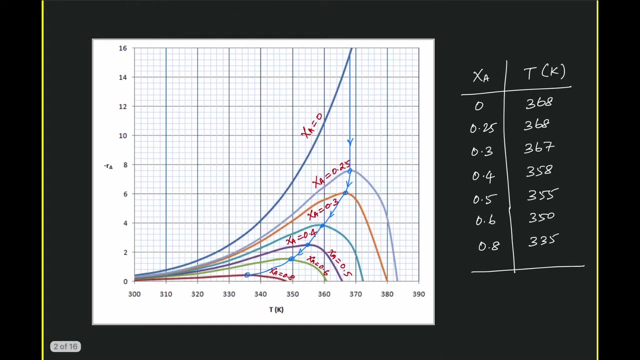 naught and xa, and again we can assume progressively changing or is we can have choose this xa at some nice values. so for these values of xa we can get the rate calculated and this rate can be plotted as a function of temperature. here again we can get the rate calculated as a function of temperature. 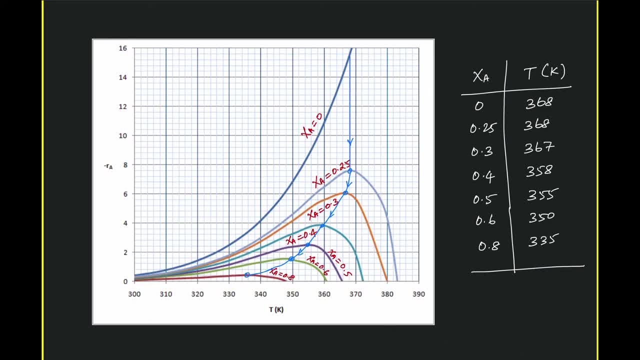 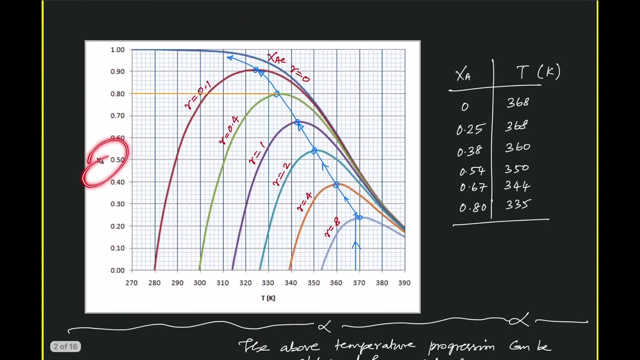 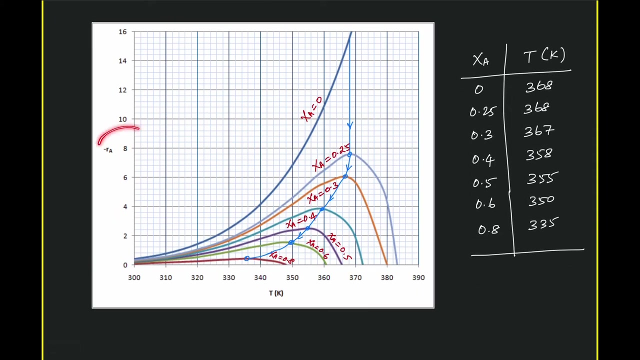 here again, the optimum temperature progression is nothing but the maxima of this xa with our rate versus temperature plot. so earlier we were having con conversion versus conversion versus temperature plot. now this is xa versus temperature plot for various rates. now we have rate versus temperature plot for various conversions. otherwise this here will be getting nice. 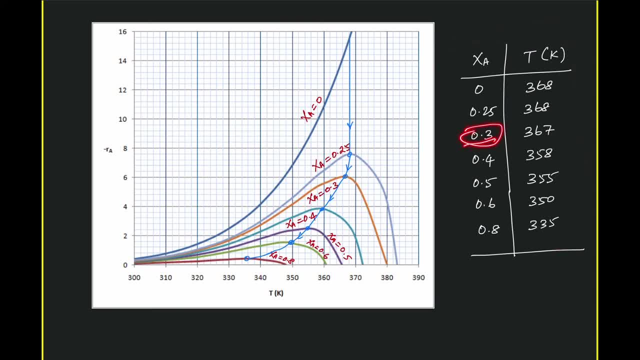 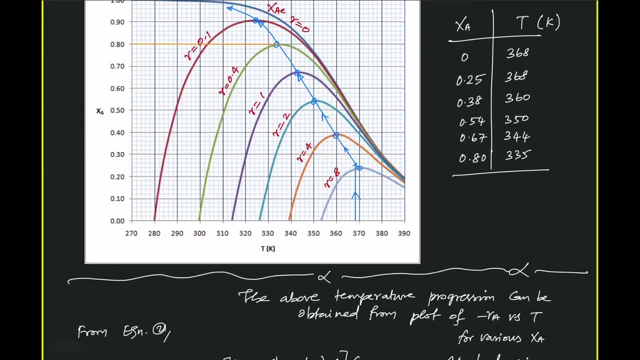 data, or is for in x, for a given conversion, what is the temperature to be operated, whereas that you cannot easily get, because we are fixing the rate and we are getting this conversion only from this maxima point, so this will be giving some 0.38. so, whereas i am interested, 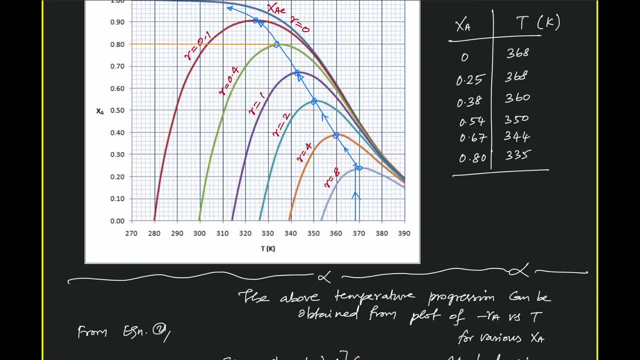 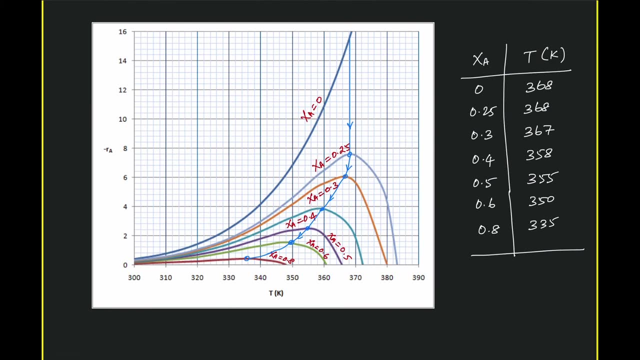 in getting the temperature corresponding to a value of 0.4, which is not readily available from this. this plot okay, so that's why we can use the plot of rate versus temperature as a function of rate versus temperature as a, with the parameters of converse conversion starting from 0.25.